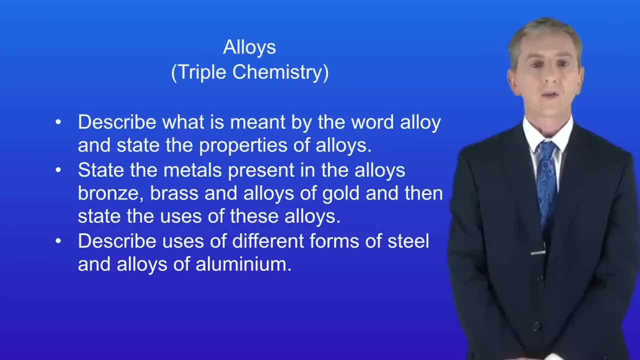 of these alloys. and finally, you should be able to describe uses of different forms of steel and alloys of aluminium. and all of this is for chemistry triple students only. So let's start by looking at the definition of an alloy. An alloy contains a metal blended with. 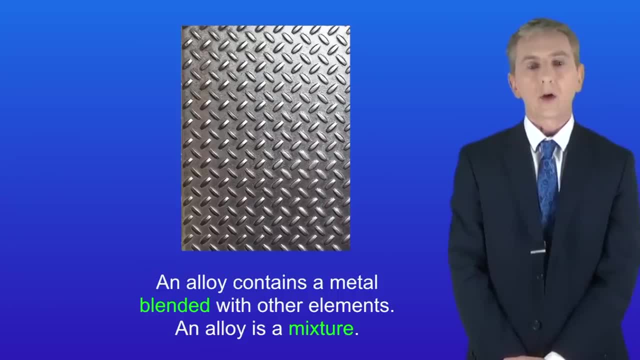 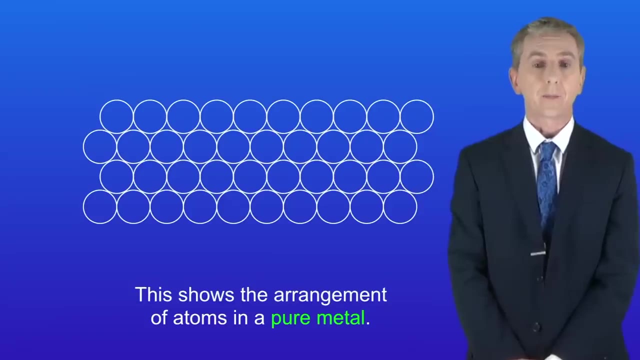 other elements. Now you need to understand that an alloy is a mixture. We make an alloy by melting our metal, mixing in other elements and then allowing the alloy to cool. Alloys tend to be harder than pure metals. I'm showing you the arrangement of atoms in a pure metal here, As: 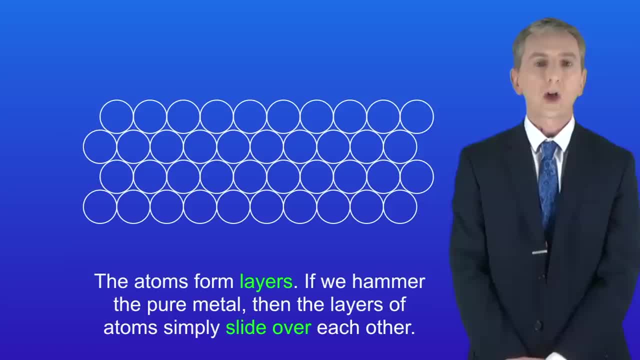 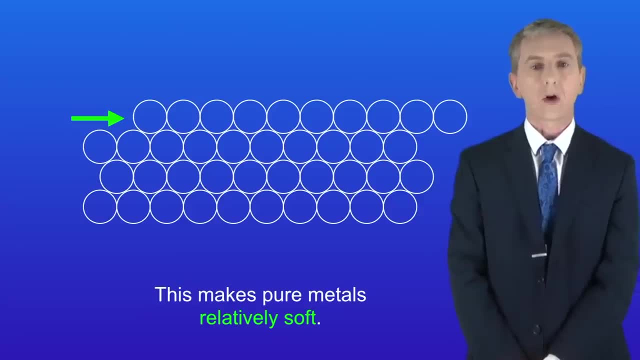 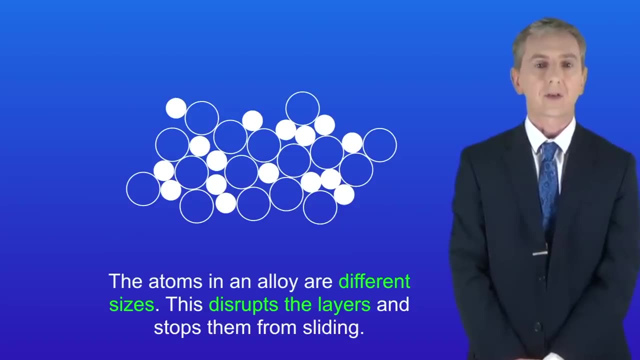 you can see, the atoms form layers. If we hammer the pure metal, then the layers of atoms simply slide over each other like this, and this makes pure metals relatively soft. This shows the atoms in an alloy. As you can see, the atoms in an alloy are different sizes. This disrupts the layers and 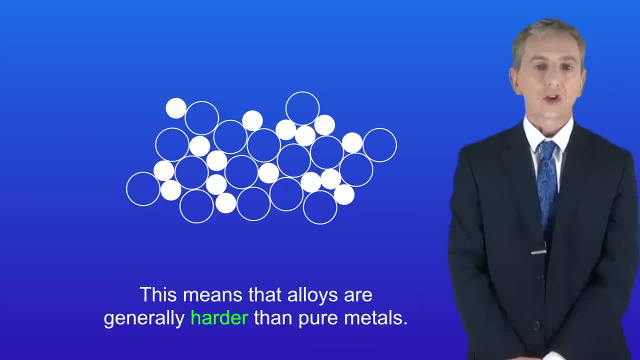 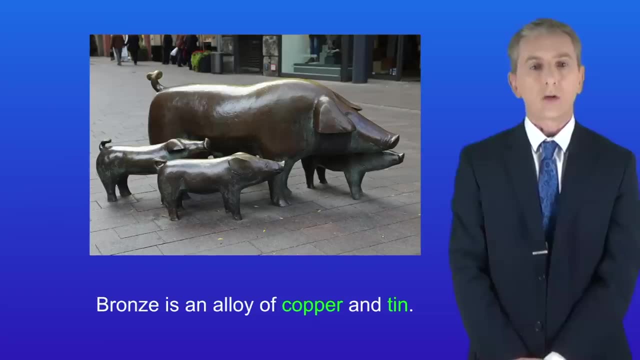 it stops them from sliding, So this means that alloys are generally harder than pure metals. We're going to start by looking at two alloys of copper. Bronze is an alloy of copper and tin. Because bronze is extremely hard and tends not to corrode, it's used for statues. 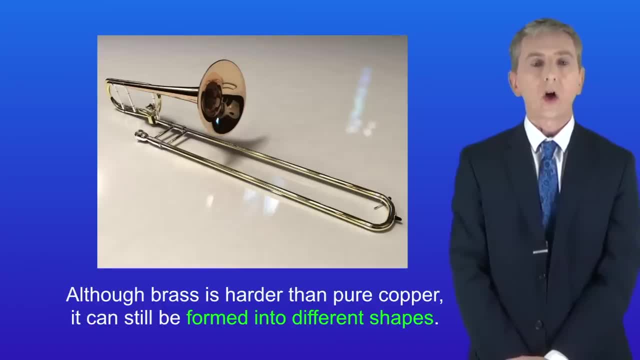 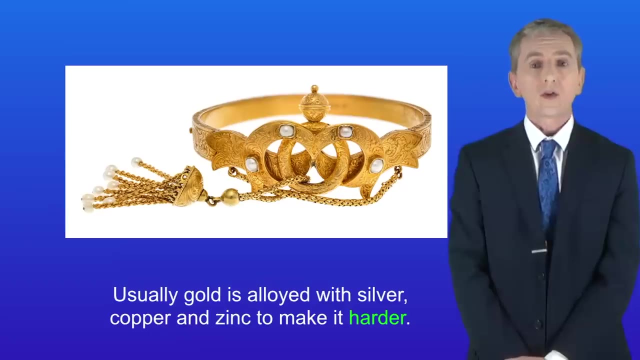 Brass is an alloy of copper and zinc. Although brass is harder than pure copper, it can still be formed into different shapes. That means that brass is used for musical instruments and door handles. Now gold is used a lot for jewellery and jewelry. But pure gold is too soft, So usually gold is alloyed with silver, copper and zinc to 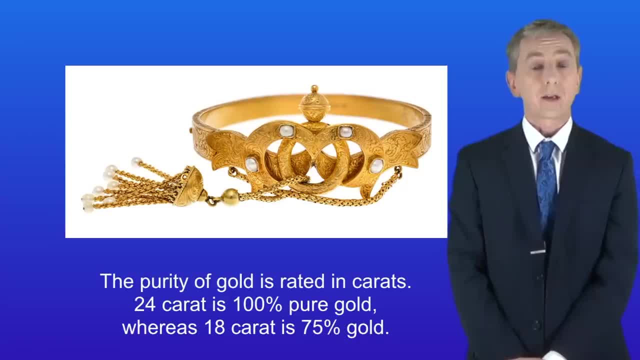 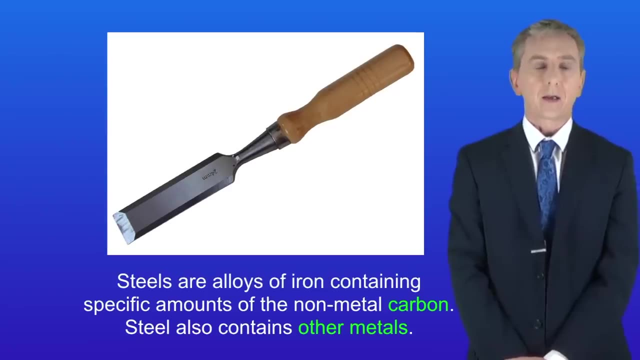 make it harder. The purity of gold is rated in carats: 24 carat is 100% pure gold, Whereas 18 carat is 75% gold. Now, one really important alloy is steel. Steels are alloys of iron containing specific amounts of the non-metal carbon. Steel also contains other metals. 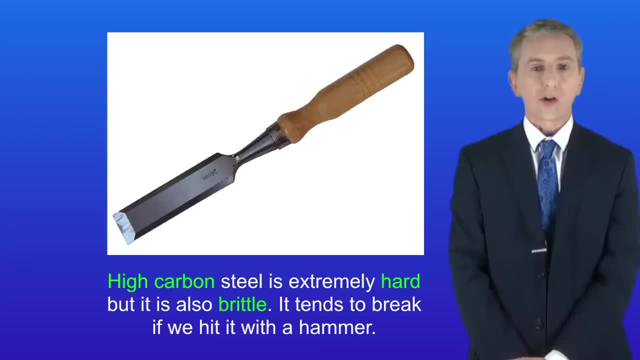 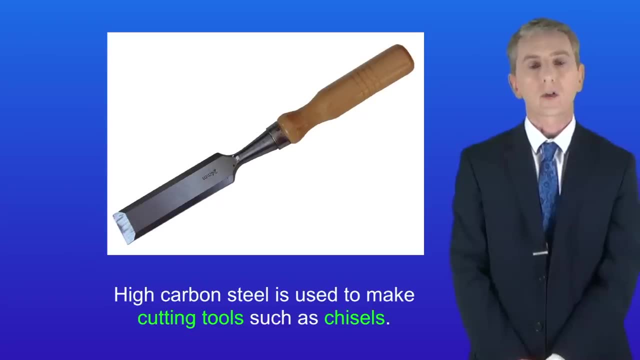 High carbon steel is extremely hard, but it's also brittle, In other words, it tends to break if we hit it with a hammer. High carbon steel is used to make cutting tools such as chisels. Low carbon steel is softer and more easily shaped. It's used to make car bodies.